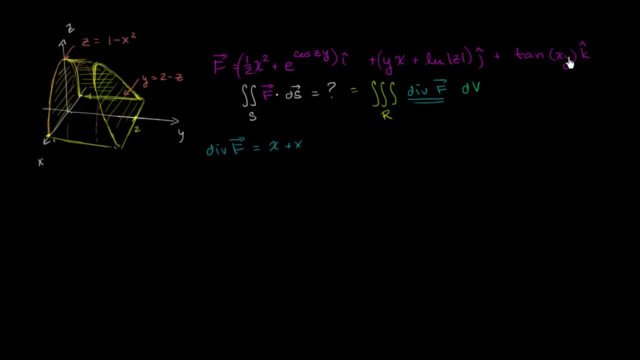 respect to y And then finally, the partial of this with respect to z. Well, this is just a constant in terms of z. It doesn't change when z changes. So the partial with respect to z is just going to be 0 here. 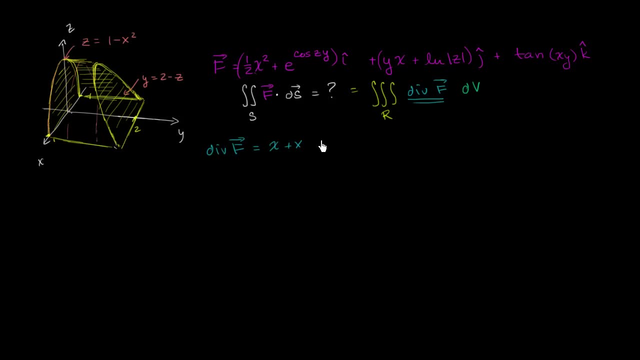 And so, taking the divergence, really, really, really simplified things. The divergence of f simplified down to 2x, And so now we can restate the flux across the surface as a triple integral. It's a triple integral of 2x. 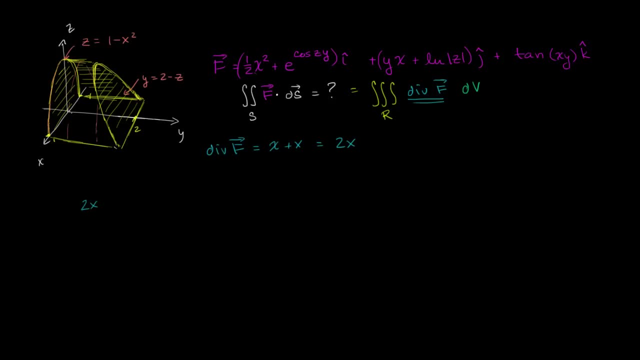 So let me just write 2x here And let's think about the ordering. So y can go between 0 and this plane. that is a function of z, So let's write that down. So y is bounded below by 0 and above by this plane, 2 minus z. 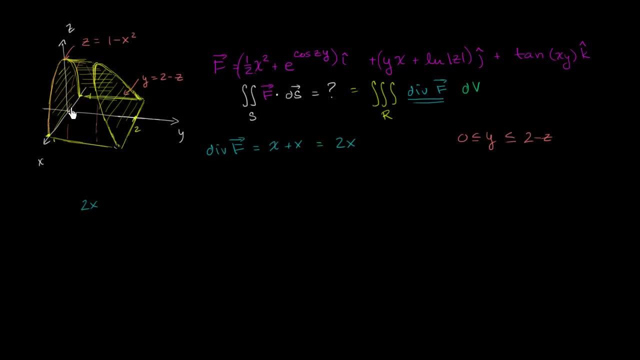 z is bounded below by 0 and above by these. you could call them these parabolas of 1 minus x squared. And then x is bounded below by negative 1 and bounded above by 1.. So negative 1 is less than or equal to x. 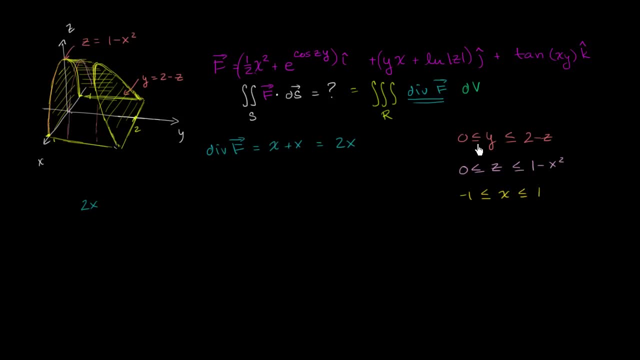 is less than or equal to 1.. And so this is probably a good order of integration. We can integrate with respect to y first, And then we'll get a function of z. Then we can integrate with respect to z And we'll get a function of x. 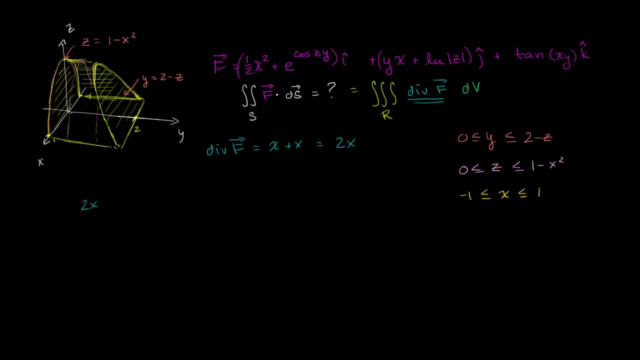 And then we can integrate with respect to x. So let's do it in that order. So first we will integrate with respect to y. So we have dy. y is bounded below at 0 and above by the plane 2 minus z. 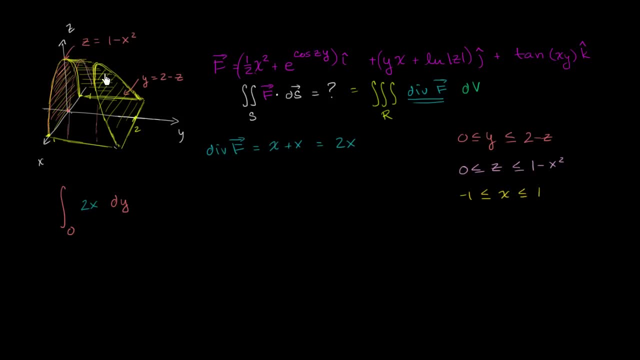 So this right over here is the plane y is equal to 0. And this up over here is the plane y is equal to 2 minus z. Then we can integrate with respect to z. Then we're going to integrate with respect to z. 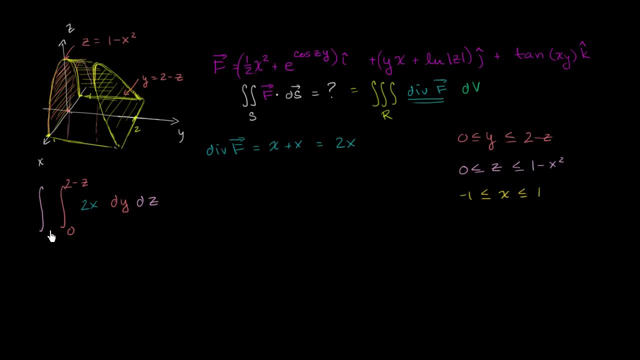 And z, once again, is bounded below by 0 and bounded above by these parabolas: 1 minus x squared. And then, finally, we can integrate with respect to x, And x is bounded below by negative 1 and bounded above by 1.. 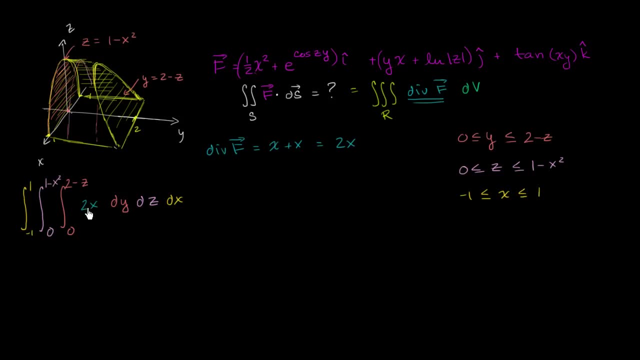 So let's do some integration here. So the first thing, when we're integrating with respect to x- sorry- when we're integrating with respect to y, 2x is just a constant. So this expression right over here, this expression right over here, 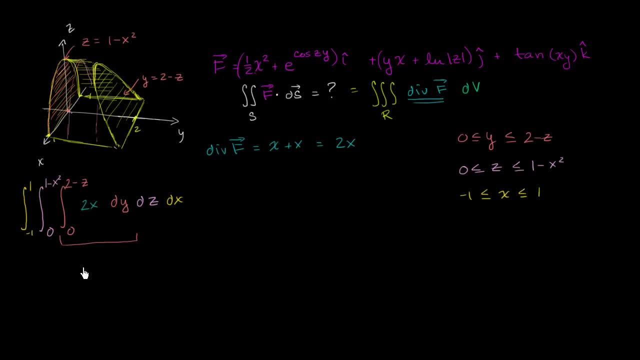 This expression right over here is just going to be 2x times y, And then we're going to evaluate it from 0 to 2 minus z. So it's going to be 2x times 2 minus z, minus 2x times 0.. 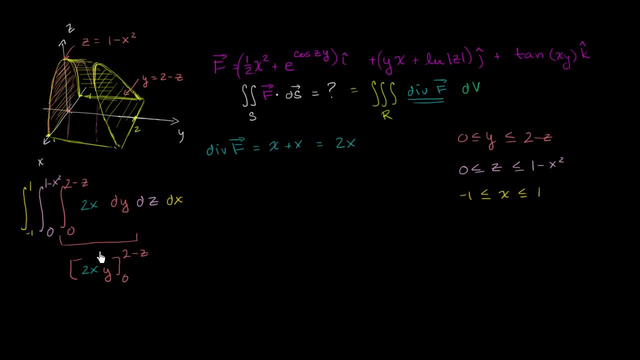 Well, that second part's just going to be 0.. So this is going to be equal to. this is going to simplify, as I'll write it this way: 2x times 2 minus z. 2x times 2 minus z. 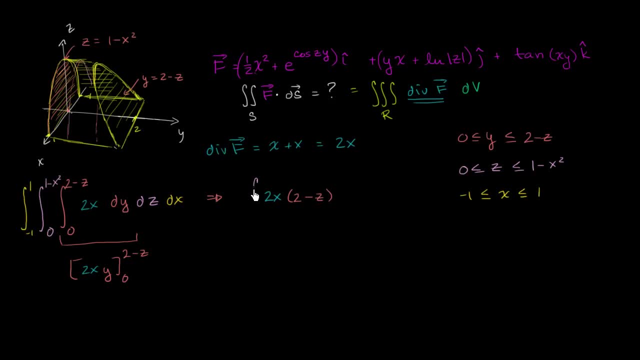 And actually I'll just leave it like that. And then we're going to integrate this with respect to z, We're going to integrate this with respect to z, And that's going to go from 0 to 1 minus x squared. 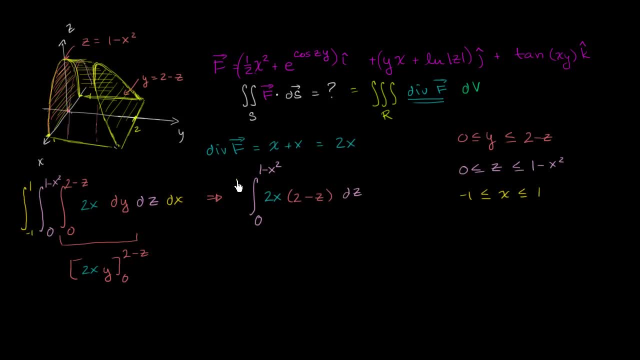 And we have our dz there And then after that we're going to integrate with respect to x: 0, sorry, negative 1, negative 1 to 1 dx: 0, sorry, negative 1, negative 1 to 1 dx. 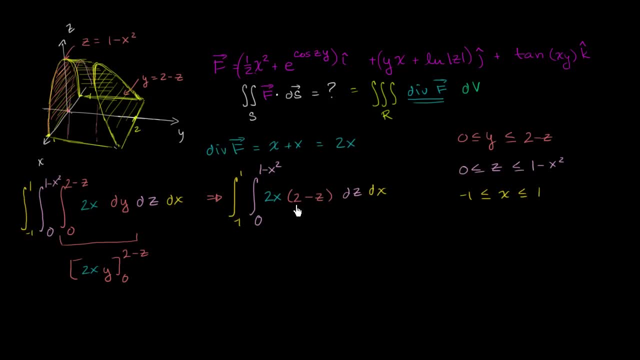 0,, sorry, negative 1, negative 1 to 1 dx. So let's take the antiderivative here. with respect to z, This you really can just view as a constant. We can actually even bring it out front, But I'll leave it there. 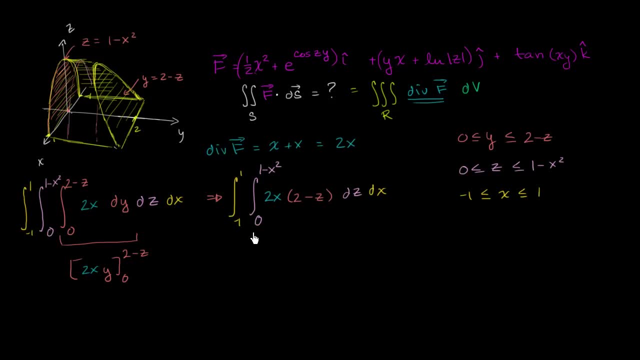 So this piece right over here- I'll do it in z's color- This piece right over here, See, we can leave the 2x out front. Actually, I'll leave the 2x out front of the whole thing. It's going to be 2x times. so the antiderivative of this. 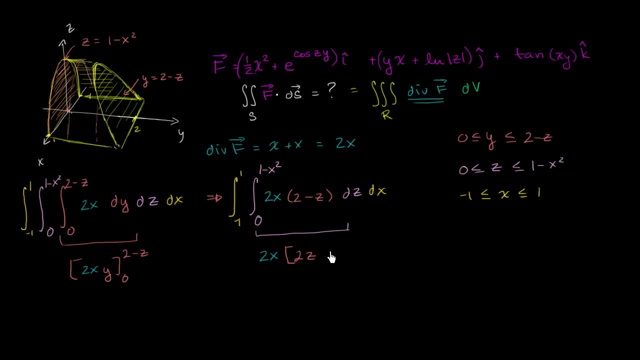 with respect to z is going to be 2z. Antiderivative of this is negative z squared z squared negative z squared over 2.. And we are going to evaluate this from 0 to 1 minus x squared. From 0 to 1 minus x squared. 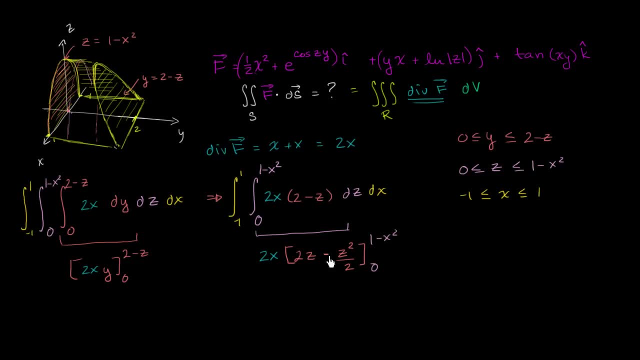 When we evaluate them at 0, we're just going to get 0 right over here, And so we really just have to worry about when z is equal to 1 minus x squared. Did I do that right? Yep, 2z and then minus z squared over 2.. 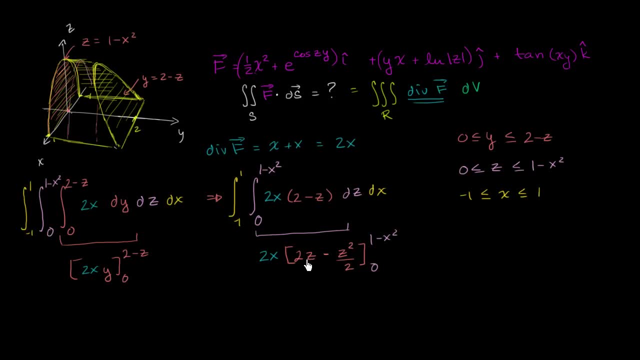 You take the derivative, You get negative z. Take the derivative here, You just get 2.. So that's right. So this is going to be equal to 2x times. let me get this right. Let me go into that pink color. 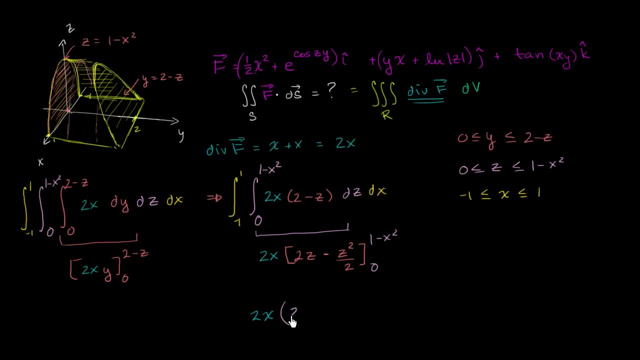 2x times 2z. Well, z is going to be 1 minus x squared, So it's going to be 2 minus 2x squared. That was just 2 times that And then minus 2x squared. 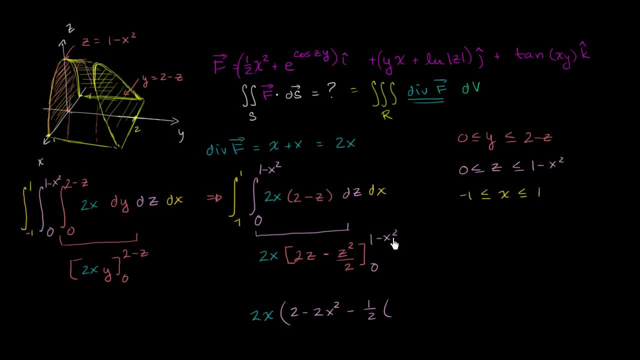 I'll just write 1 half times this quantity squared. So this quantity squared is going to be 1 minus 2x squared plus x to the fourth. That's just some basic algebra right over there, And then from that you're going to subtract. 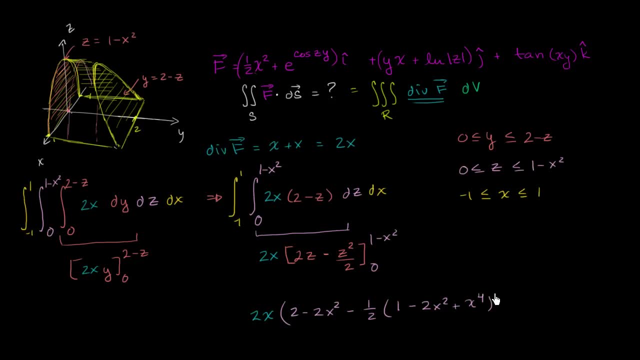 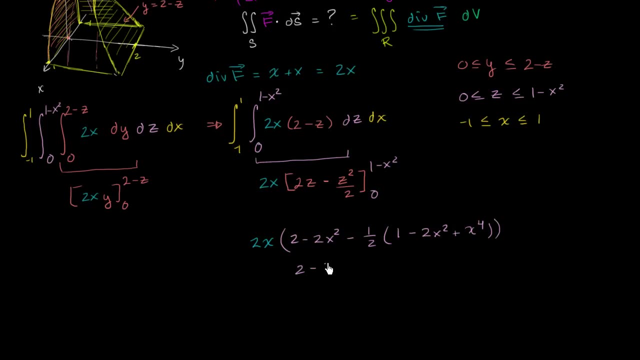 this thing evaluated at 0, which is just going to be 0. So I just won't even think about that. And now we need to simplify this a little bit And we are going to get: if we simplify this, we get 2 minus 2x. 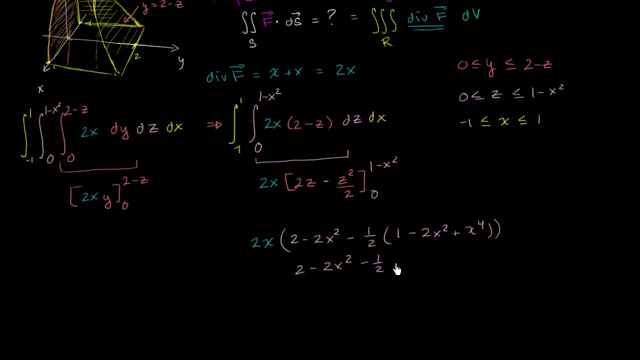 squared Minus 1 half And then plus, so this is negative 1 half times negative, 2x squared. So it's going to be positive x squared minus 1 half x to the fourth. Let's see, can we simplify this part? 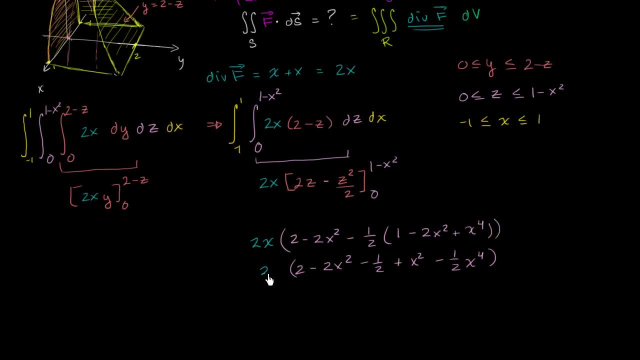 Let me just make sure we know what we're doing here. So we have this 2x right over there. I want to make sure I got the signs right. Yep, looks like I did. And now let's look at this. Let's see. can I simplify it a little bit? 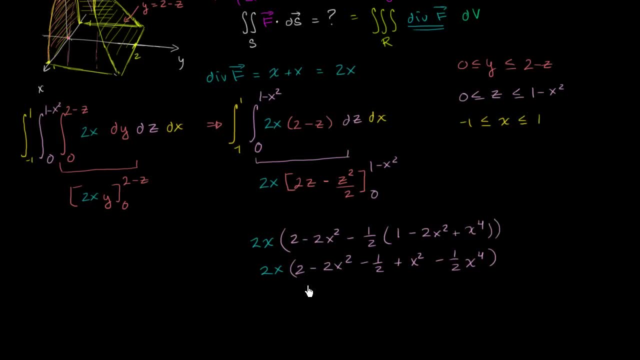 I have 2 minus 1 half Minus 1 half, which is 3 halves. So I have 3 halves, That's that term, and that term taken into account. And then I have negative 2x squared plus x squared. 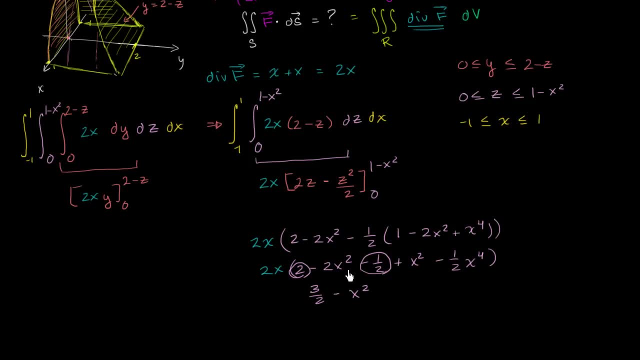 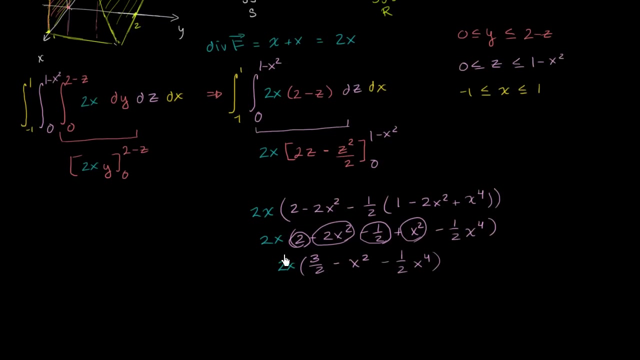 So that's just going to result in negative x squared if I take that term and that term, And then I have negative 1 half x to the fourth And I'm multiplying this whole thing by 2x, And so that's going to give us 2x times 3 halves. 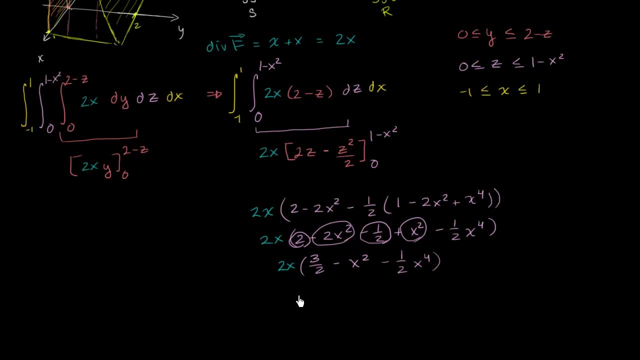 And I want to make sure I'm doing this slowly so I don't make any careless mistakes. The 2's cancel out, You get 3x And then 2x times negative. x squared is negative, 2x to the third. 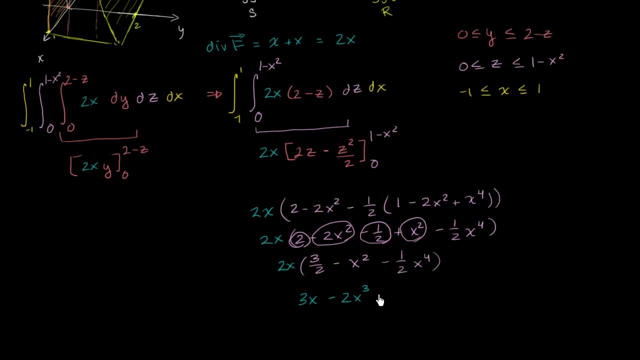 And then 2x times this right over here. The 2 cancel out with the negative 1 half. You have negative x to the third, Minus x squared, minus x squared, minus x to the fifth. So all of this simplifies to this right over here. 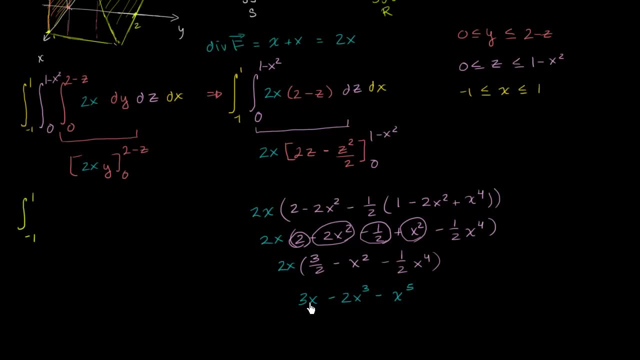 So our whole thing simplifies to an integral with respect to x. x will go from negative 1 to 1 of this business of 3x minus 2x to the third, minus x to the fifth, And then we have dx, And now we just take the antiderivative. 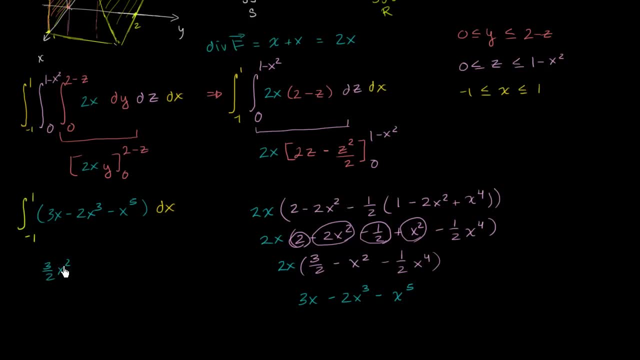 with respect to x, which is going to be 3 halves, x squared minus x squared Minus, let's see, to the x to the fourth, power Minus 1 half, because it's going to be 2 fourths x to the fourth. 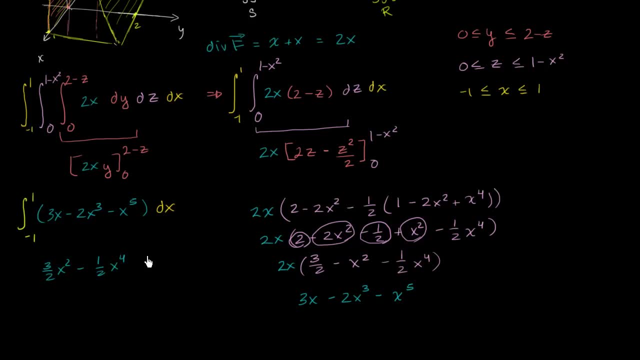 Is that right? Because if you multiply it you're going to get 2. Yep x to the third And then minus x to the sixth, over 6. And it's going to go from 1 to negative 1. Or negative 1, negative 1 to 1.. 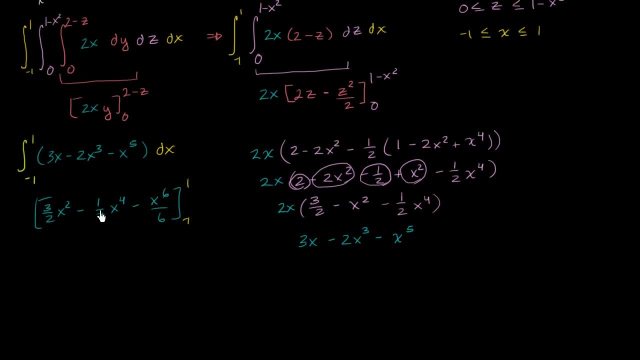 So when you evaluate it at 1, I'll just write it out real fast. So first, when you evaluate it at 1, you get 3 halves minus 1 half minus 1 half, Plus 1 sixth, And then from that we are going to subtract 3 halves minus 1 half. 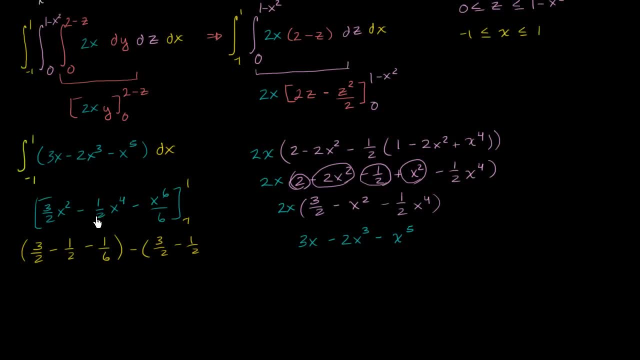 plus 1 sixth, Or actually no, they're actually all going to cancel out. Is that right? Are they all going to cancel out? Yep, I think that's right. They all cancel out. So it's actually going to be plus. or I should say: 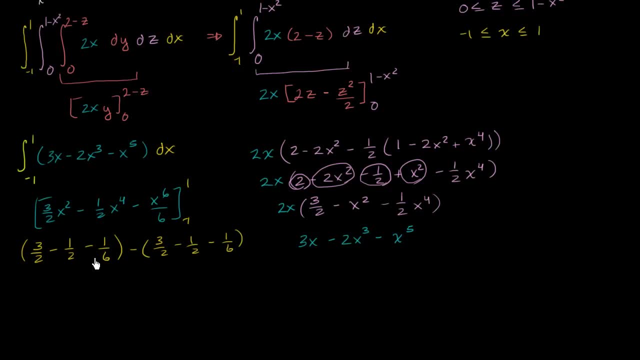 minus 1 sixth right over here, And then all of these cancel out. That cancels with that. That cancels with that Because we're subtracting the negative 1 half, And that cancels with that, And so we are actually left with 0..